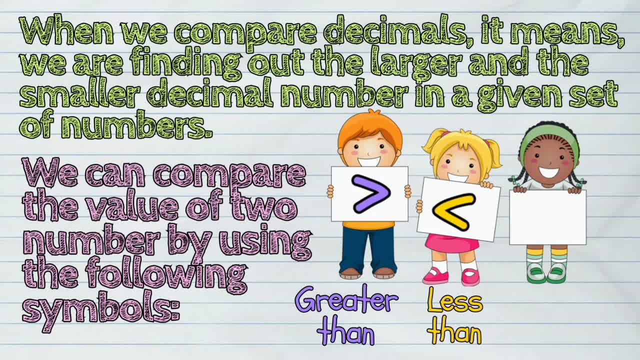 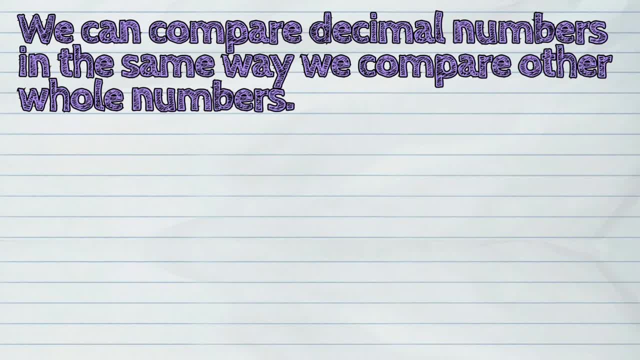 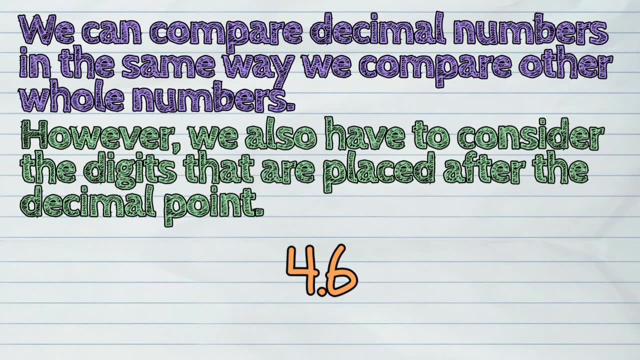 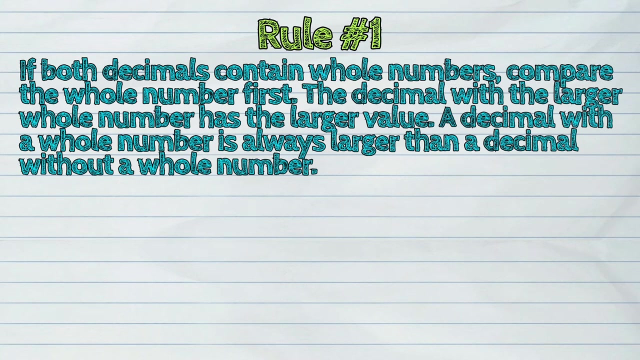 Greater than, less than and equal to. We can compare decimal numbers in the same way we compare other whole numbers. However, we also have to consider the digits that are placed after the decimal point. Let us study these following rules First. if both decimals contain whole numbers, compare the whole number first. 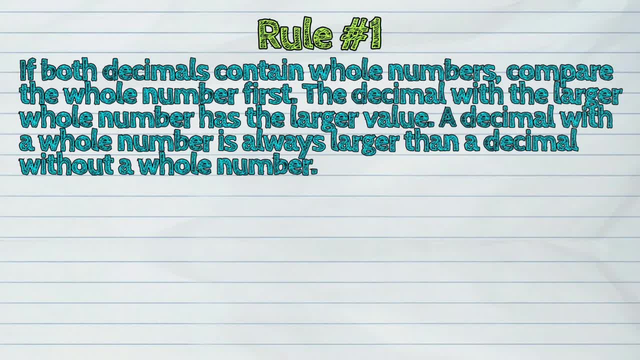 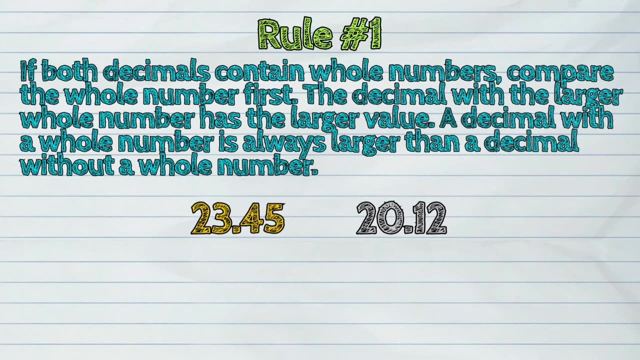 The decimal with the larger whole number has the larger value. A decimal with a whole number is always larger than a decimal without a whole number, Like this example: 23 and 45. 25 hundredths is greater than 20 and 12 hundredths, since the whole number 23 is larger than 20.. 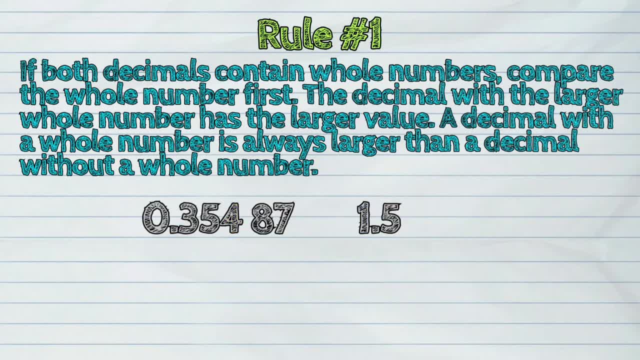 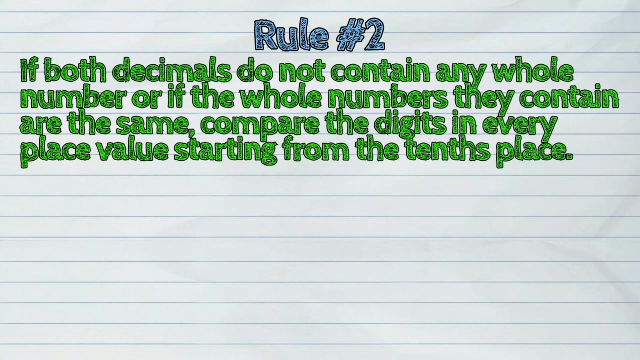 Another example: 35,487 hundred thousands is less than 1 and 5 tenths because it has no whole number compared to the other. Let us now proceed to the second rule: If both decimals do not contain whole number or if the whole numbers they contain are the same. 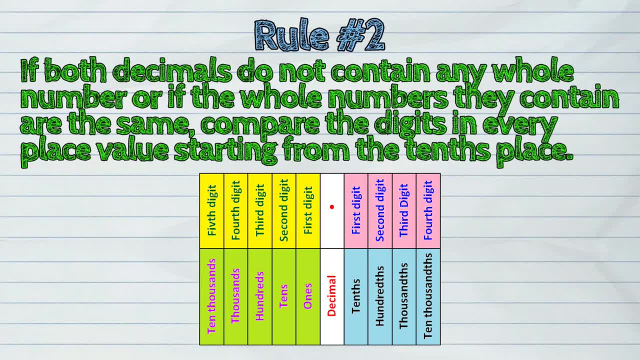 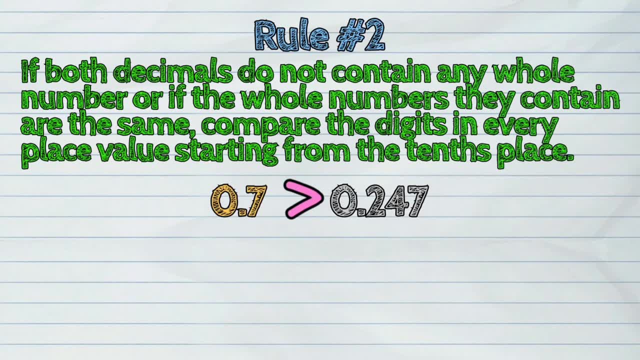 compare the digits in every place value starting from the tenths place: 7 tenths is greater than 247 thousandths, Because we should compare first the value in the tenths place, which are 7 and 2.. 7 is greater than 2.. 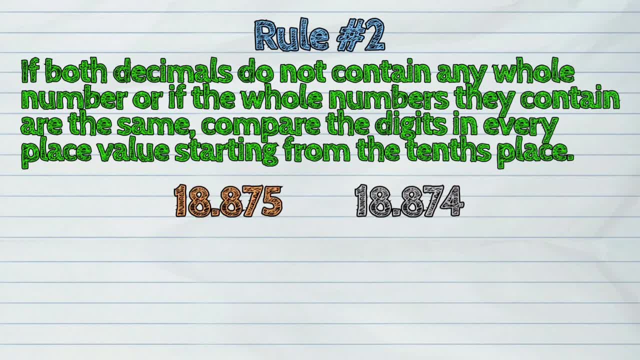 Another example: 18 and 875 thousandths is greater than 18 and 874 thousandths Because in this case We are comparing the value in their thousandths place. Five thousandths here is greater than four thousandths. Now let us proceed to the third rule.